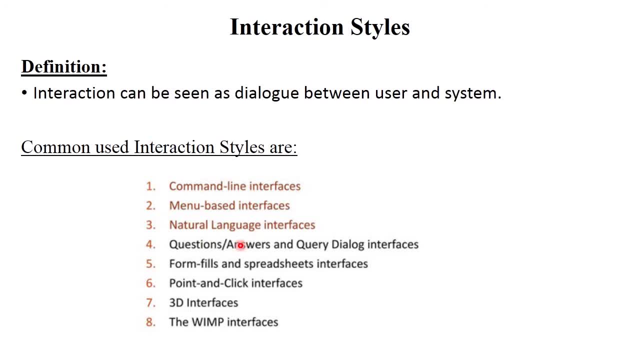 and query dialogue interface. These four interaction style I already explained in my previous video. Now in this video we will learn about form fills and spreadsheet interface, point and click interface, 3D interface and WIMP interface. These eight are the common used interaction. 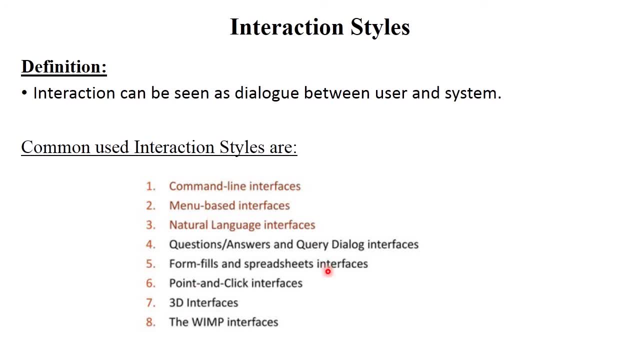 style Means by using these softwares or by using this application, we are able to create a common use interaction style. Now in this video, we will learn about form fills and spreadsheet interface, point and click interface, 3D interface and WIMP interface. These eight 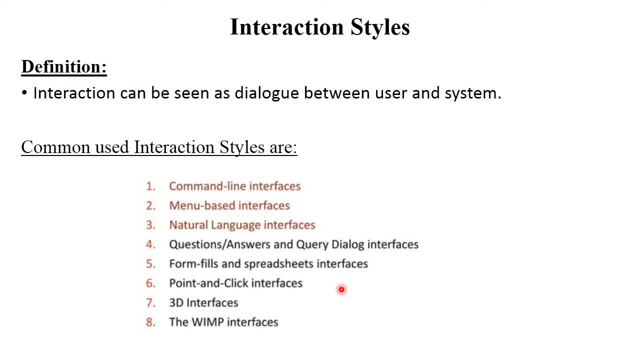 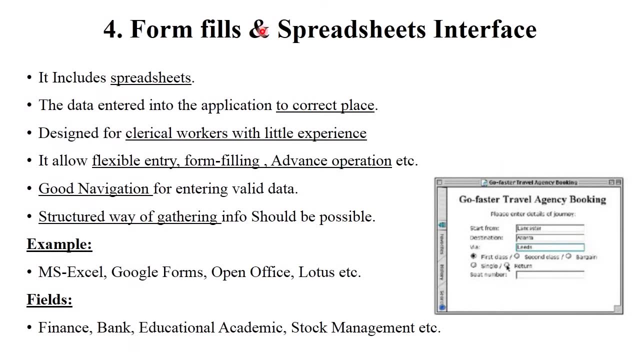 are the common used interaction style Means. by using these softwares or by using this application, you have to interact with computer or the system Clear. So let's see first, form fills and spreadsheet interface Next. So we all are familiar with form fills and 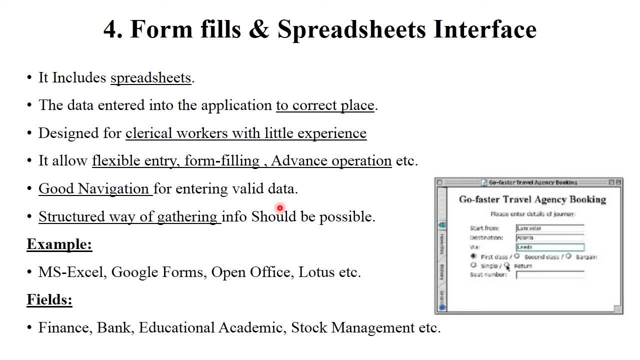 spreadsheet interface. We all used Microsoft Excel. We should fill different forms online. So these all are examples of spreadsheet interface: The data entered into the application up to the correct place. in Microsoft Excel There is tabular format in rows and columns format data. If there is a particular column, for example age, So you have to enter the age. 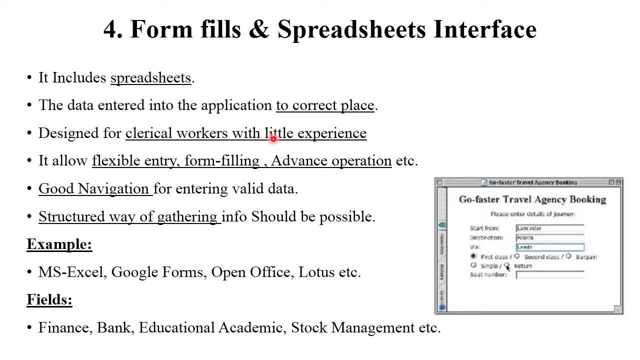 in positive format or in positive integer number. for Right, Suppose there is a, a column mobile number, So you have to enter 10 digit mobile number only in that particular column. So Microsoft Excel required good navigation for entering valid data. So afterciu it is. 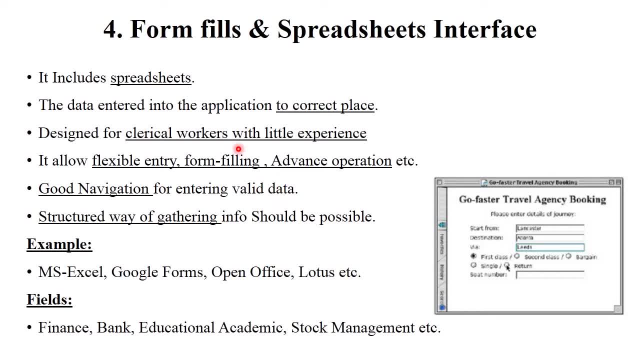 working now and synagoguecom For more information. read by touching theœt link in description only. so each and every generation, whether it is technical people and non-technical people, used microsoft excel or online forms. filling are little experiences, so it is designed for clerical workers with more experience. the microsoft excels or spreadsheets have structured format. 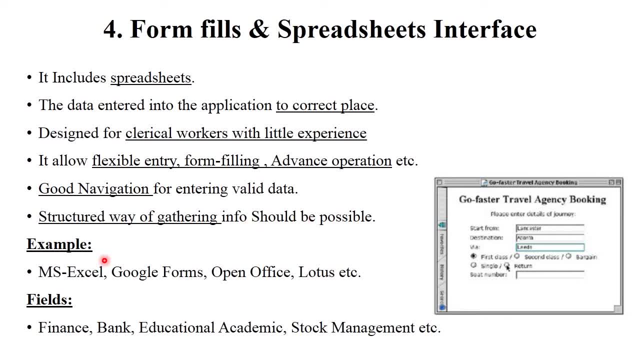 it gathering information. it should be possible. the examples are microsoft, excel, google forms, open office, lotus, etc. lotus is generally used with linux for storing data and spreadsheets have flexible entry. you have to enter as per amount of data, as per the column or in structured format. 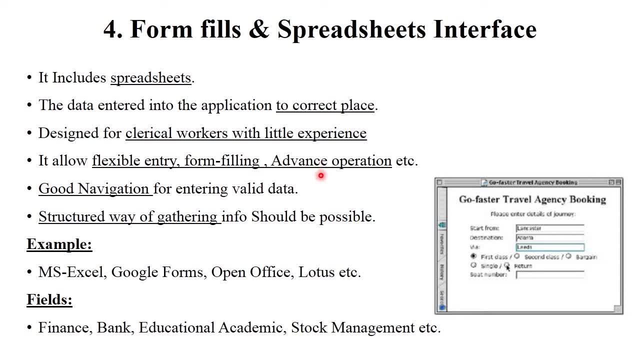 there are different advanced operations, form fillings also available. there are different fields where used spreadsheets, like finance, bank, educational, academic stock management, etc. generally each and every field for, for, for. for storing data in particular format we have to use microsoft excels or different forms clear. the another example is form filling. so this is just example, like go faster travel agency. 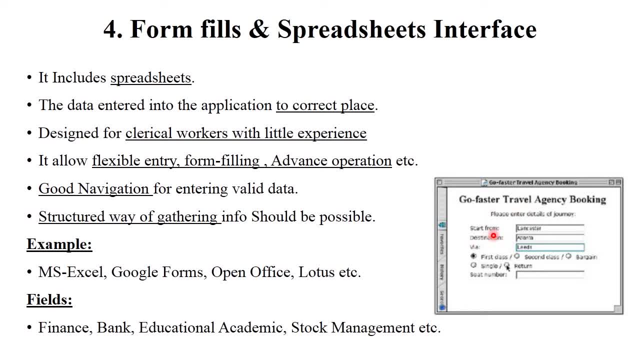 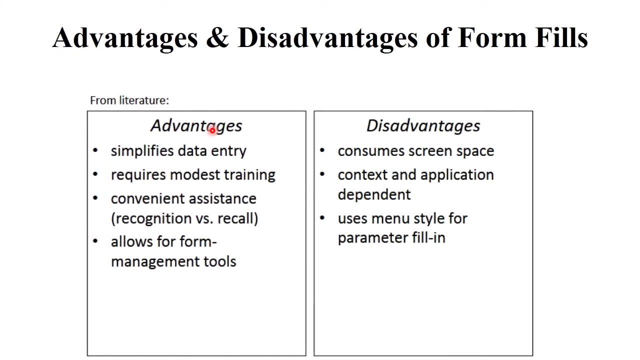 booking. so there is start from means, destination and starting place, the your class, first class, second class- and their ticket single or return seat number. so this is a particular online form for travel agency booking. so this is also an example of form filling server volleyball. i would have sugar. 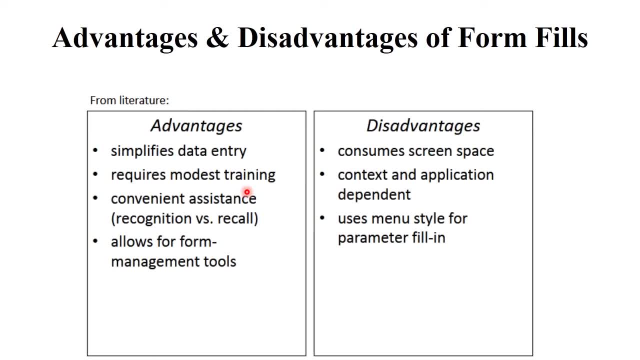 training if you use different type of database, like Microsoft SQL or I can. so for the database or storing information in database you have to require proper training training. but for microsoft excel it requires modest training. convenient assistant, you can easily use it and allow for form management tools clear. the disadvantages are: it consumes screen space. in microsoft excel there are so. 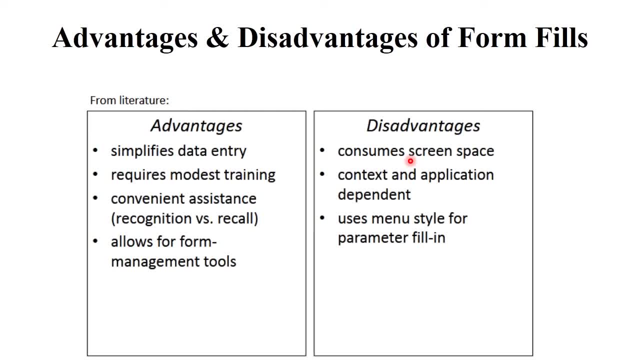 many columns and rows so it consumes the screen space clear, then context and application dependent. if you uh required large amount of data, so microsoft excel is not suitable for that, or because it required a large amount of time for filling the information sometime only. okay, so as per the requirement, as per your requirement, you have to use different database or you have to use 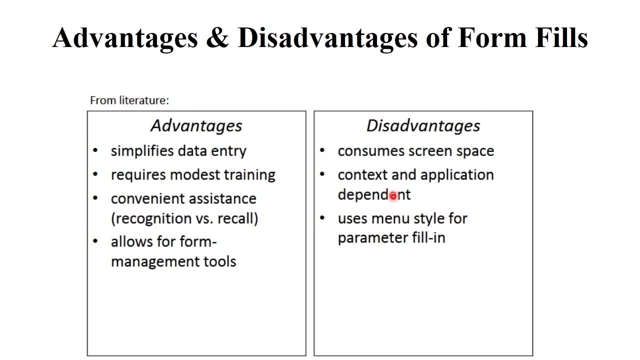 microsoft excel. it completely depends on your requirement. it uses menu style for parameters. there are different menus are available. sometimes there are tricky options or different formulas, like some as well. average. this kind of formulas are available. so, as per your knowledge, as per your requirement, you have to choose which type of files or database used for storing information. clear next, the next. 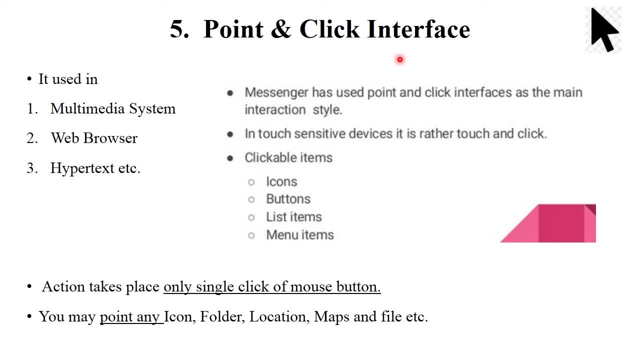 interaction style is point and click interface. we all are familiar with that. the point and click interface generally used in multimedia system, web browser, hypertext, etc. pointer simply means literally click, sign okay, by using mouse you have to click on each and every folders. the action takes place only single click of mouse button. you may point any icon, folder, location, maps, files, etc. 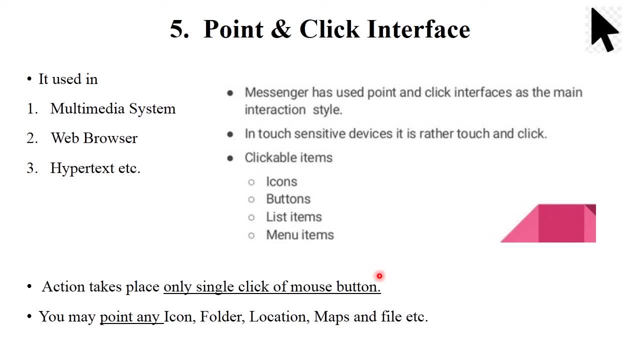 clear. for double click you have to open a new folder clear. so this is the point and click interface. messenger has used to. point and click interface is the main interaction style. when you type a message there is one particular vertical line for right. so this is the point and click interface. there are various clickable. 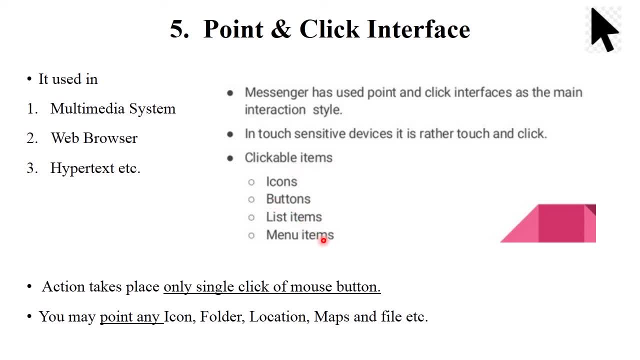 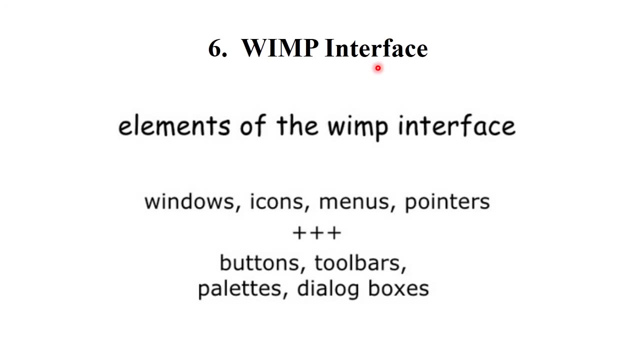 items like icons, buttons, list item, menu items, etc. it touch sensitive device. it is rather touch and click clear. so we all are familiar with this point and click interface. next, the next one is WIMP interface. so first, what is mean by WIMP, the elements of WIMP? W stands for windows, I stand for icons, M stands for 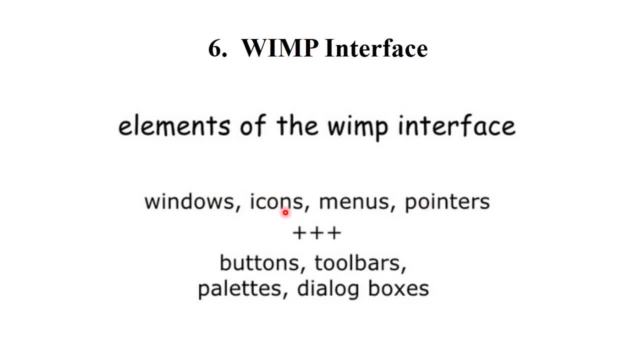 menus and P stands for pointers, windows icons, menus and pointers. these are called as WIMP interface. we again all are familiar with that. we have to use a different Windows system, like computers, mobiles. each and everyone has particular screen right. different types of icons are available on that, different types of menus available on that right. so by using 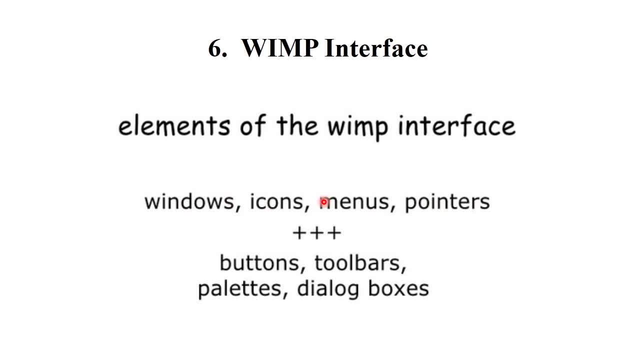 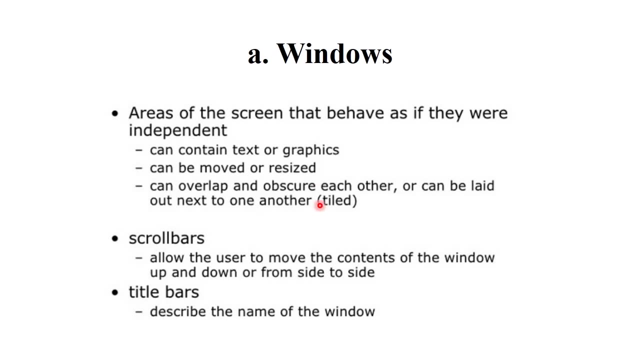 pointers. you have to use different icons, menus, folders, etc. so this is called as WIMP interface, or WIMP interface is generally available on each and every device. clear next. so let's see in detail, one by one. the first one is windows. we all are familiar with windows. windows means area of the screen that behaves as: 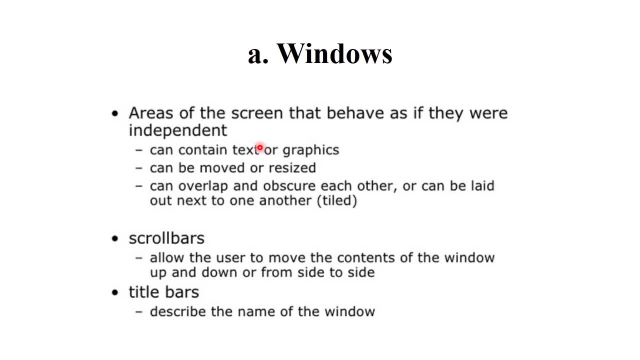 if they were to be used as a screen, they would be used as a screen, and they would be used as a screen if they were independent. there is particular independent screen of each and every device, either it is computer or mobile, etc. so this windows screen content different text or graphics sometimes. 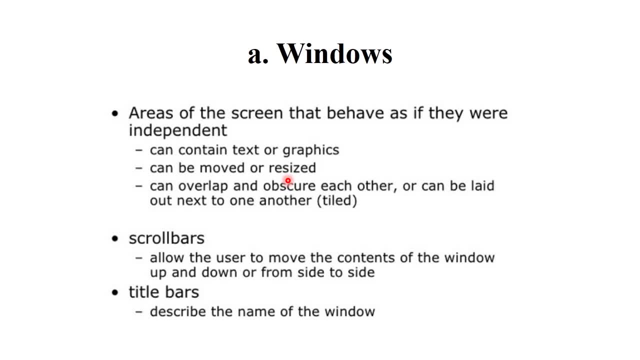 windows screens are: move or resize. you have to minimize it, maximize it, etc. right, there are different scroll bars and title bars also available. scroll bars means it move the content from window up and down, like a page up and down. this kind of functionalities also available. clear then title bar. title bar: describe the name. 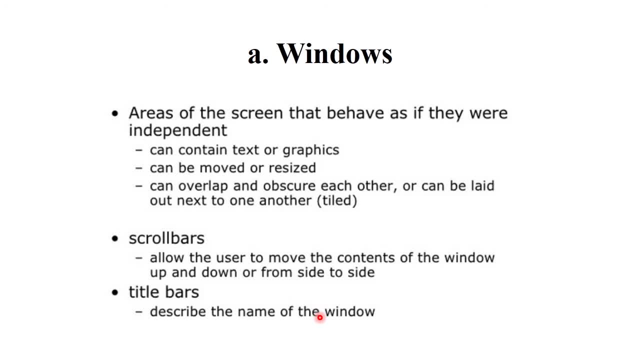 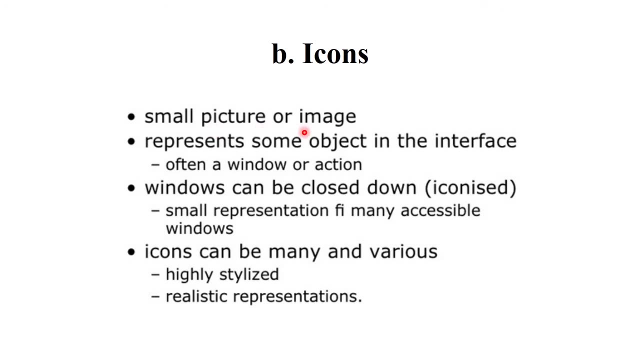 of the window. there is different title bars also available. clear. so this: all types of information is available directly on window and we all are familiar with that. clear. the next one is icon. icon means generally small picture or image. it represent the object in that particular interface. see, there are different types of social apps available, like whatsapp, facebook, insta, right. so 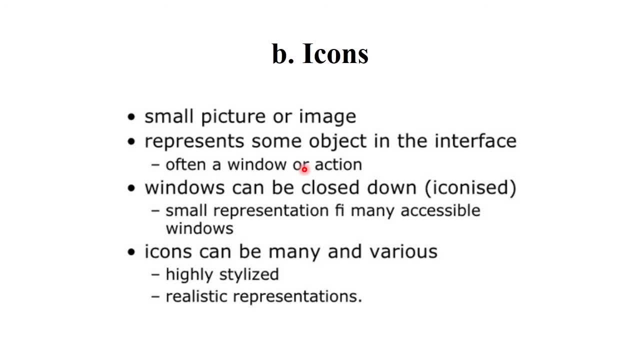 each and every applications has different icons so it easy to identify. there are different: mozilla, firefox, chrome, internet explorer, opera, so all are browsers, but there are different. icons are present so we can easily find out which types of browsers there are. clear so windows can be closed down or 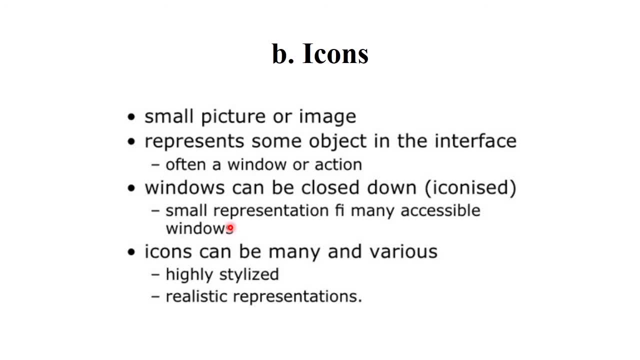 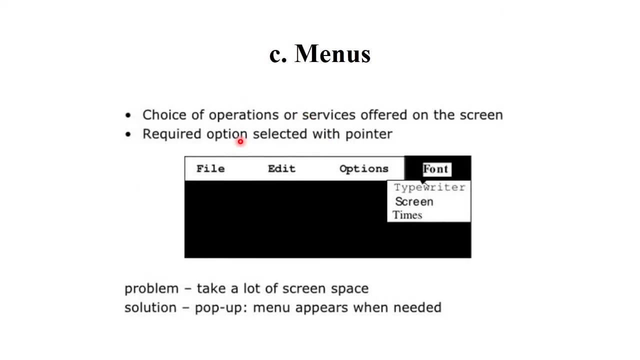 using icons. it's a small representation of many accessible windows. icons can be many and various format: clear: it shows the realistic representation or highly stylized. okay, next one is menu. again, we all are familiar with the menu option. menu means choice of operations or services offered on the screen. it required option selected with pointer. so, for example, see: 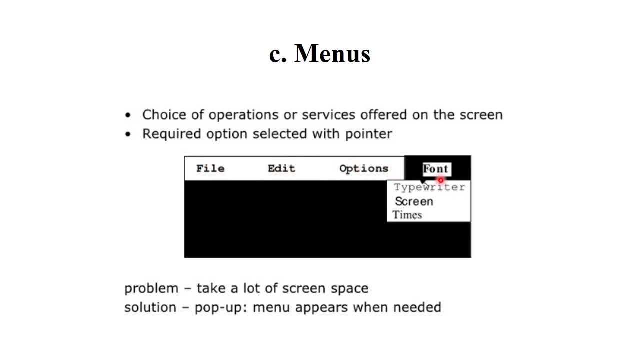 here there are different menus available like file edit option, font by using pointer. if you click on that there are again different cascading menu like typewriter screen times. this kind of functionality is available, clear. so this is menu, but problem is it take a lot of screen space sometime. there are different. 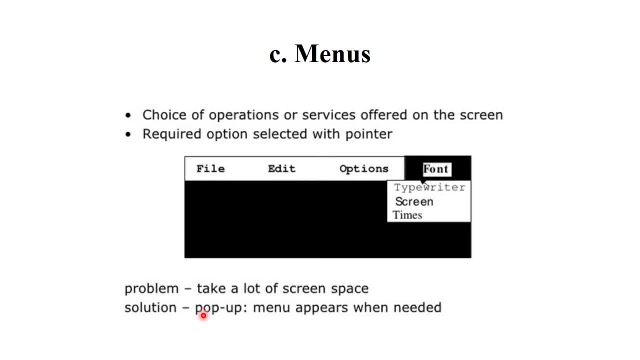 types of menus are available on this screen, so the solution is pop-up menu. it appears when needed. okay, so if there is file menu, in file there is new, or in edit, in edit there is cut copy paste. this kind of option is available, so it may help us in à little bit as a page.